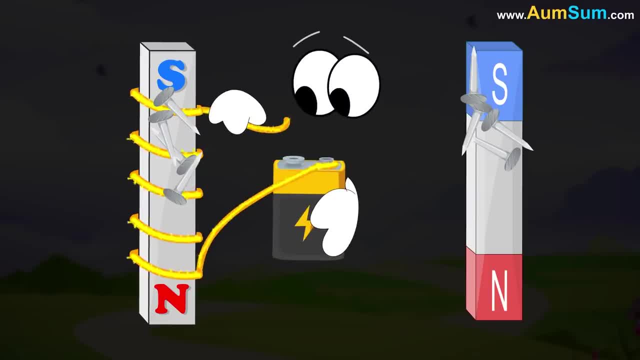 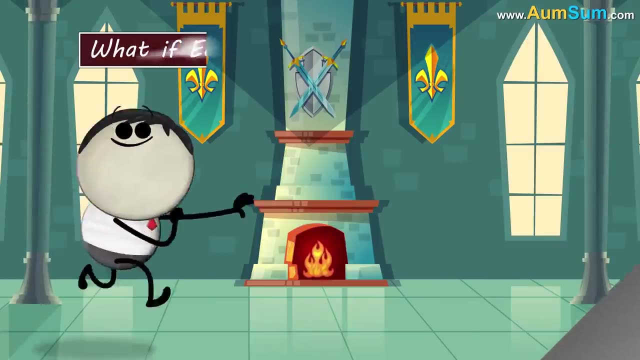 The only difference is that the magnetism is not permanent. Once the current is removed, magnetism may stop working suddenly or after some time. An electric bell is a good example of the use of an electromagnet. What if earth's magnetic poles flipped? 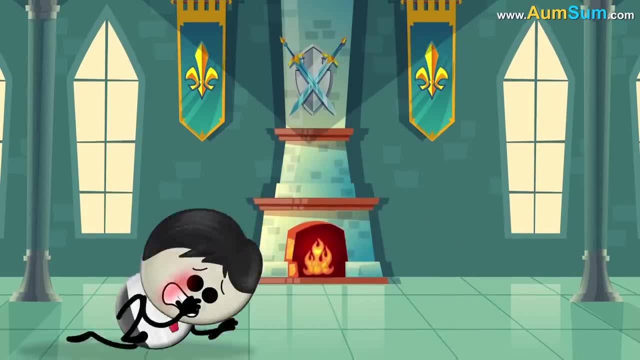 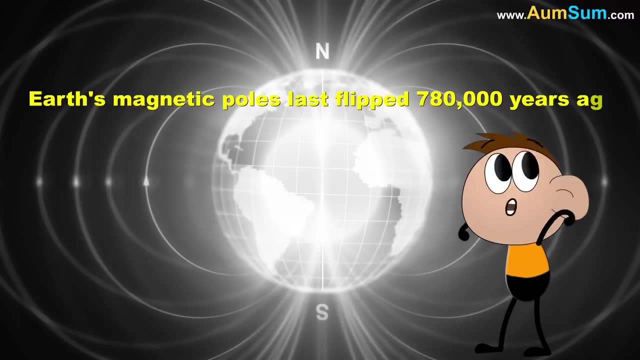 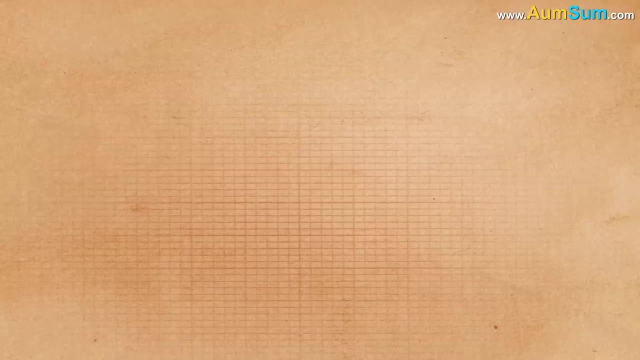 Then I will perform A backflip. Wow AumSum, Earth's magnetic poles last flipped 780,000 years ago. If it were to flip now, following problems might occur: Firstly, Greenland will end up in the southern hemisphere, While Antarctica in the northern hemisphere. 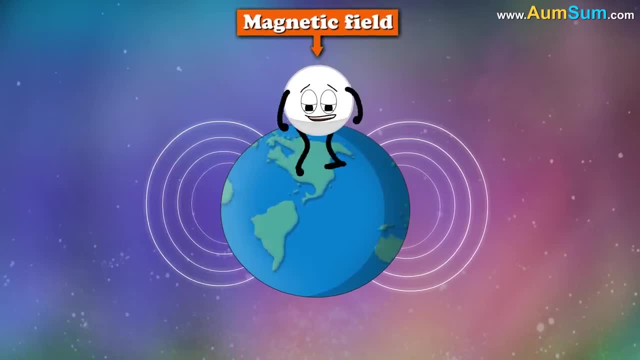 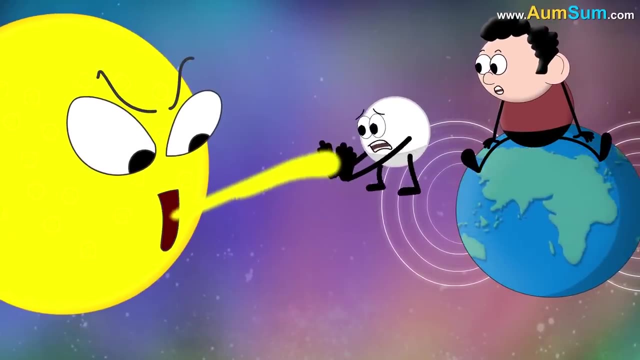 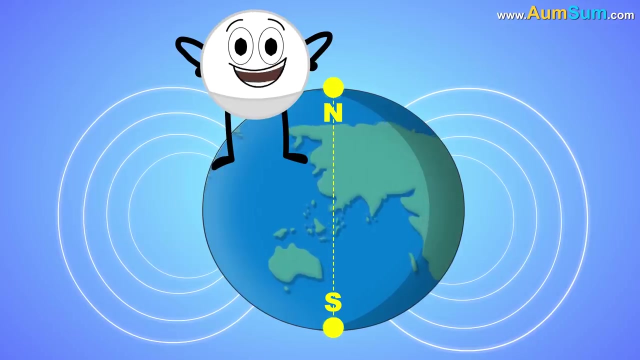 Secondly, scientists believe that earth's magnetic field gets weaker before flipping. Now, magnetic field protects us From harmful solar winds, Hence its weakening might cause serious health consequences. Thirdly, scientists also believe that, before flipping, The weak magnetic field leads to the creation of multiple north and south poles on earth. 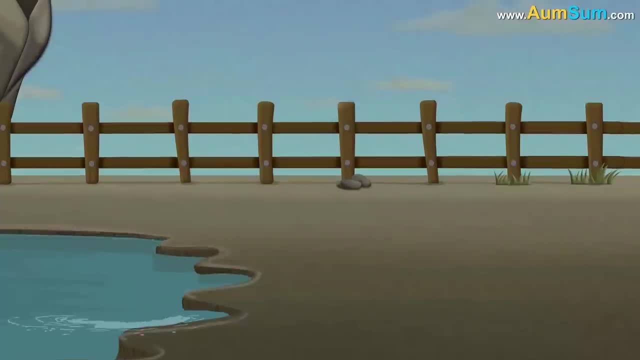 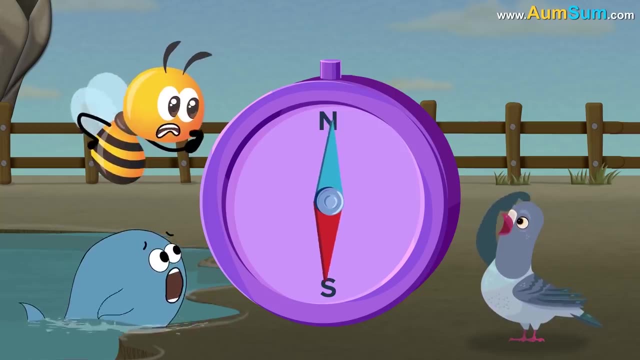 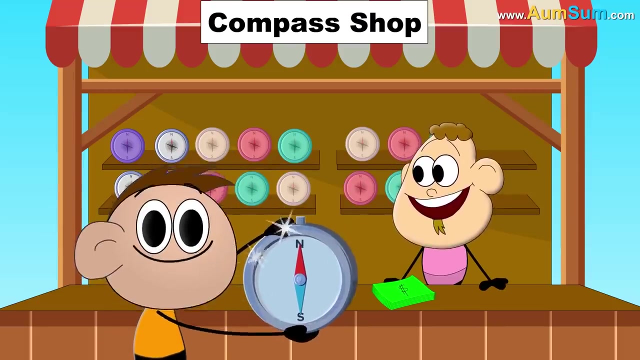 For a short period of time. Fourthly, species such as pigeons, whales, bees, etc. Which rely on the magnetic field for navigation will get disoriented. Lastly, we will definitely need to buy a new compass. What if magnets disappeared? 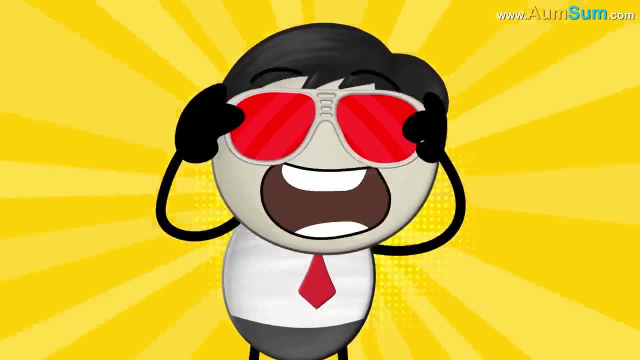 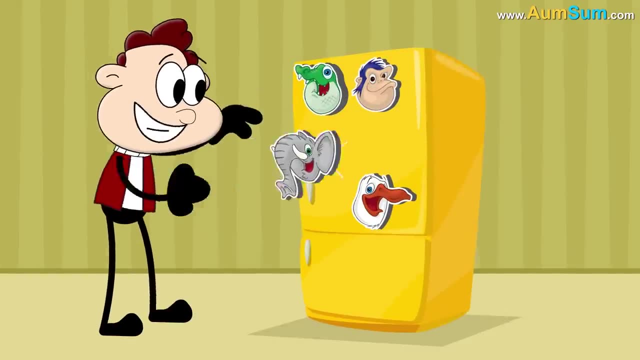 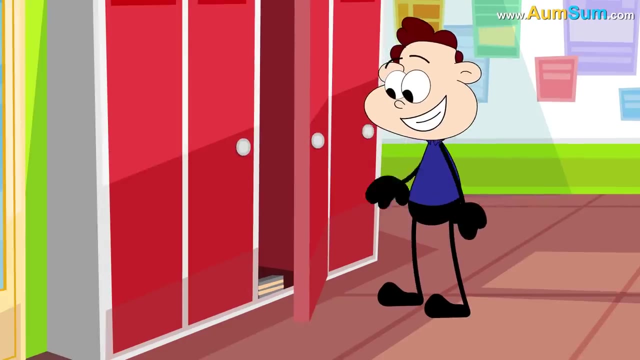 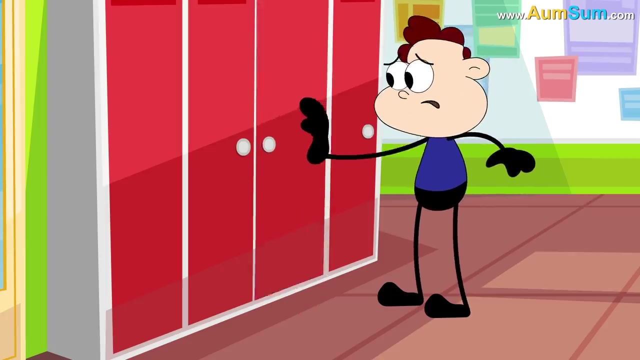 No problem, I have a magnetic personality, Oh AumSum. Firstly, if magnets disappeared, People who love to put magnetic stickers on fridge would be extremely disappointed. Secondly, magnetic latches are used to firmly close cupboards. If magnets disappeared, cupboards may not close that well anymore. 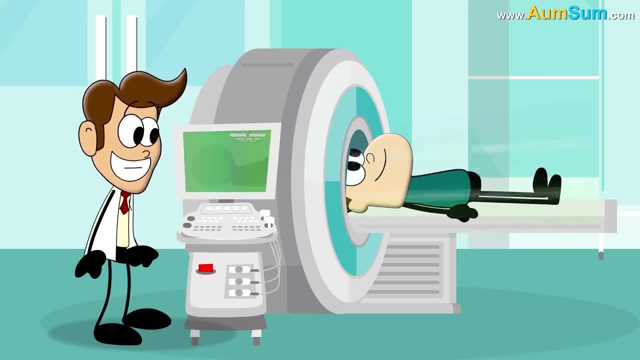 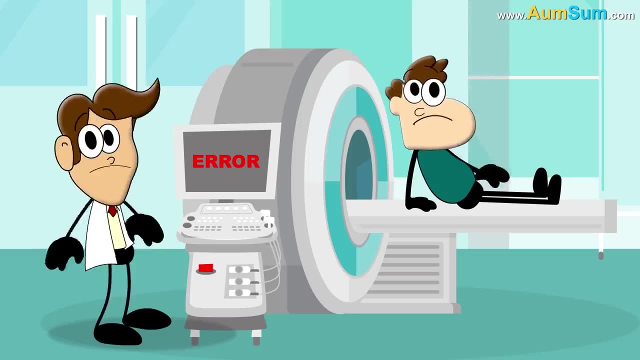 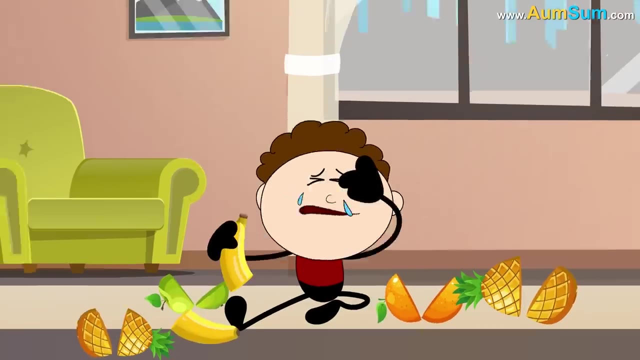 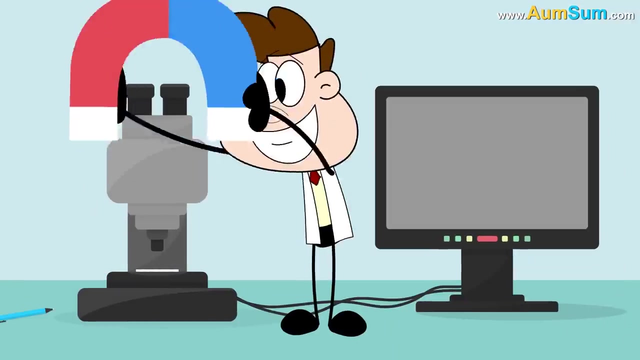 Thirdly, MRI machines use extremely strong magnets. If magnets disappeared, doctors as well as patients would be extremely disappointed. Fourthly, magnetic toys are popular among kids. If magnets disappeared, parents may face a tough time keeping their kids entertained. Lastly, magnets are required in many scientific experiments. 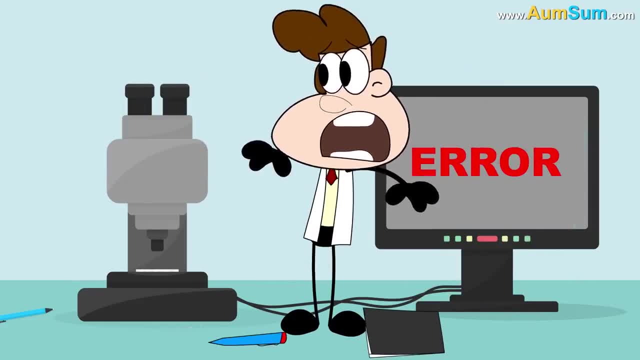 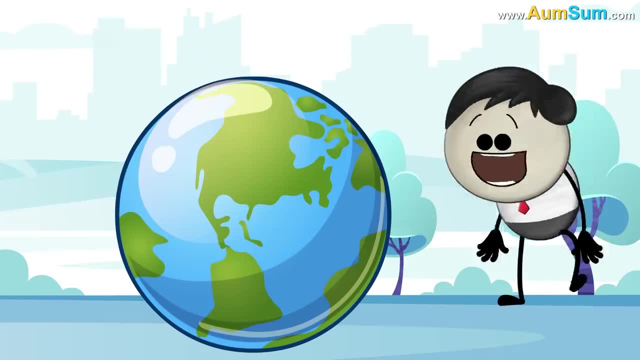 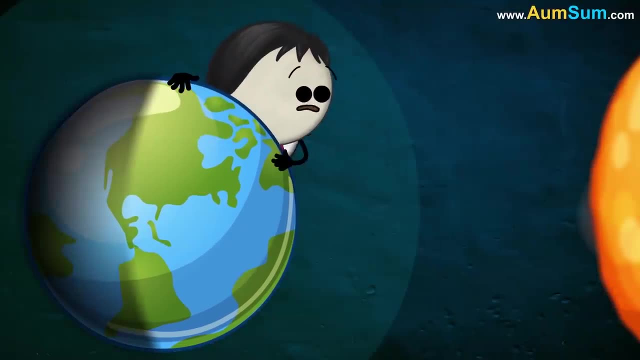 If magnets disappeared, scientists would be one sad lot. Why is equator hot but poles are cold? Because equator likes hot burgers and poles like cold burgers? No, Firstly, around the equator, sun rays hit the ground at a 90 degree angle. 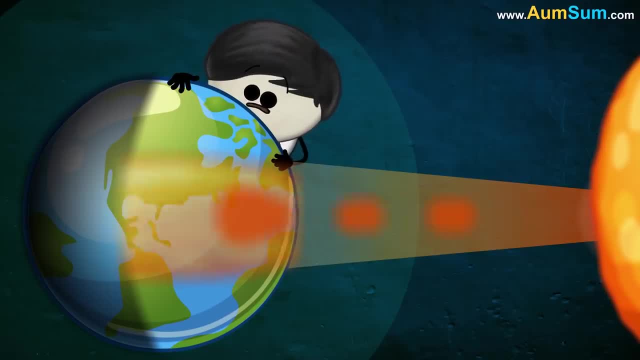 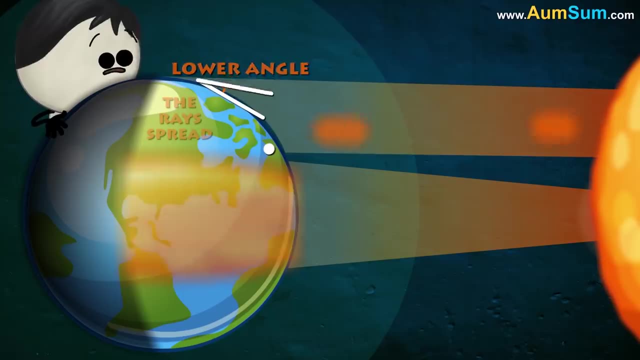 Hence, more solar energy falls per unit area, Thus making equator hot. However, near the poles, since sun rays hit the ground at a lower angle, The rays spread, causing less energy to fall per unit area, Thus making poles cooler. 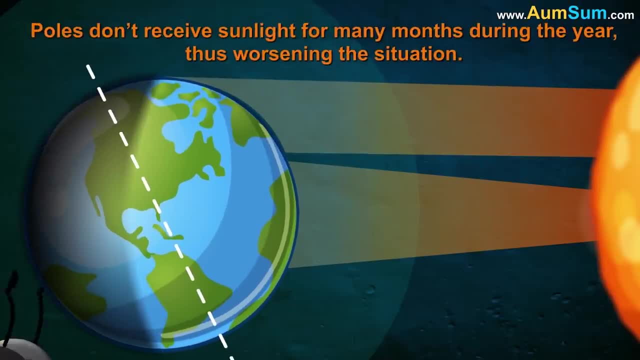 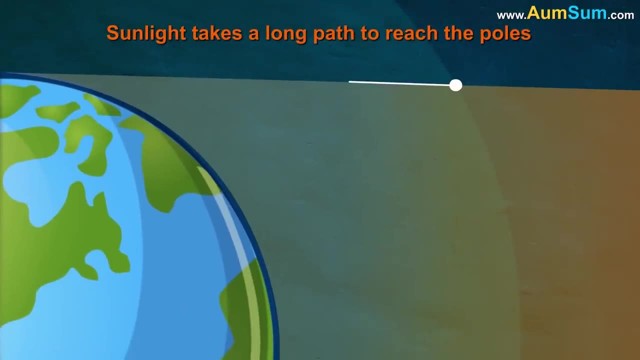 Secondly, due to the earth's axial tilt, poles don't receive sunlight for many months during the year, Thus worsening the situation. Thirdly, as sunlight takes a long path to reach the poles, It has to deal with a greater number of atmospheric particles. 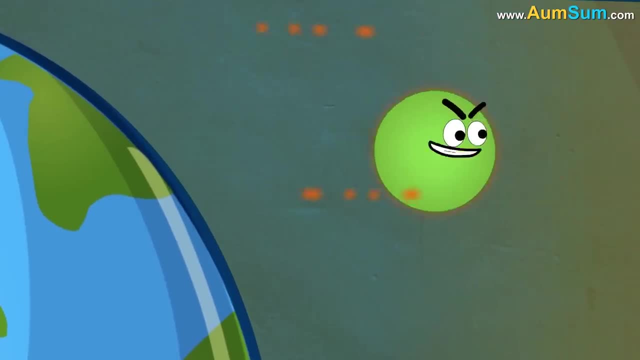 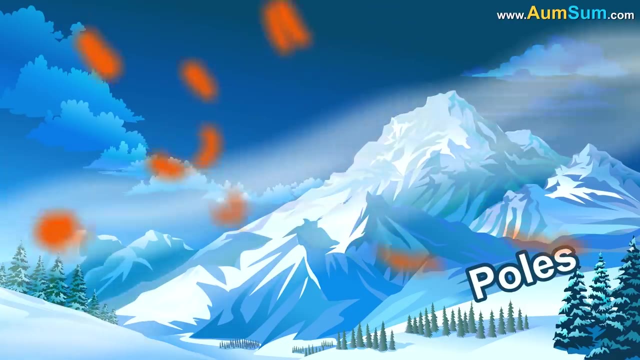 Which results in more absorption and scattering And scattering of sunlight. Thus less sunlight reaches the poles. Lastly, snow at the poles reflects 75 to 95% of sunlight, Which is much more as compared to that reflected by the land around the equator. 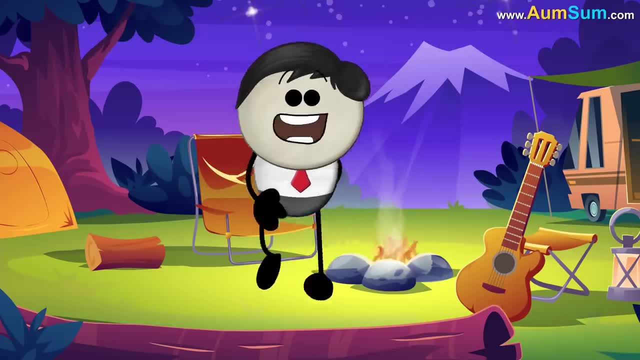 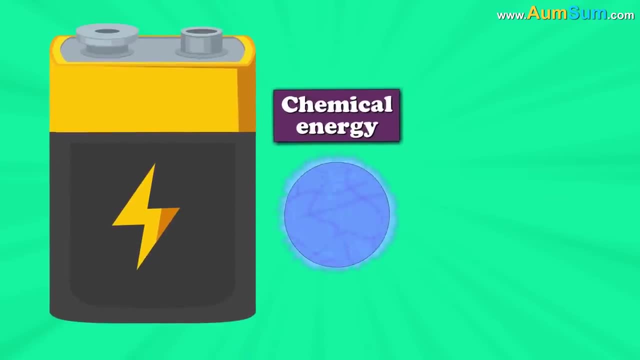 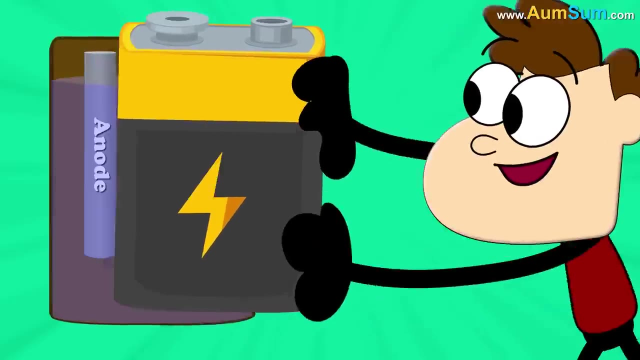 How do batteries work? That is a secret I can't tell anyone. A battery works by converting chemical energy into electricity. A battery consists of one or more electrochemical cells. An electrochemical cell consists of two electrodes separated by an electrolyte. 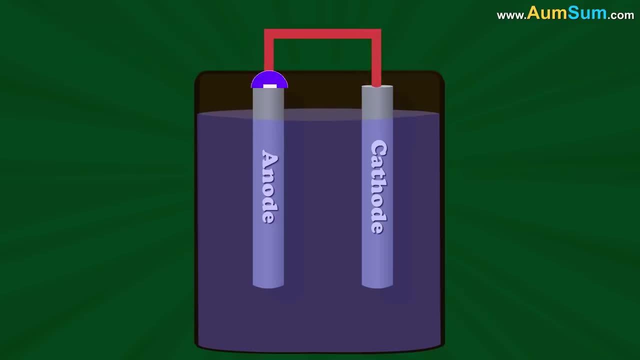 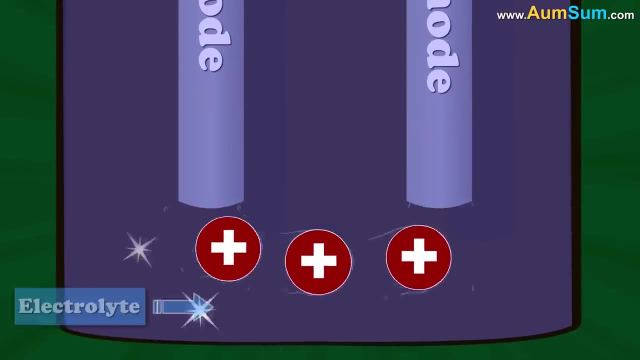 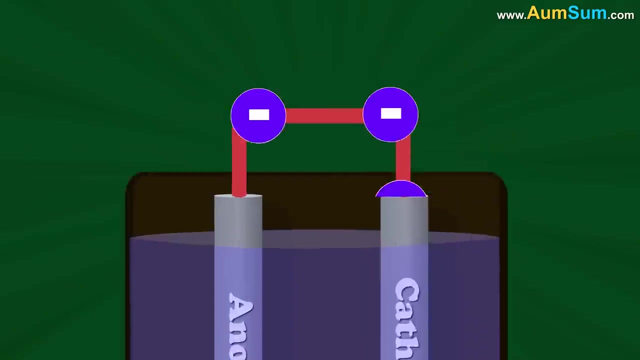 When the battery's two electrodes are connected into a circuit, The negatively charged electrons start flowing through the external wire, While the positively charged ions start flowing through the electrolyte. This balancing of charge is important to keep the reaction running. Now, this flow of electrons through the external wire is basically electricity. 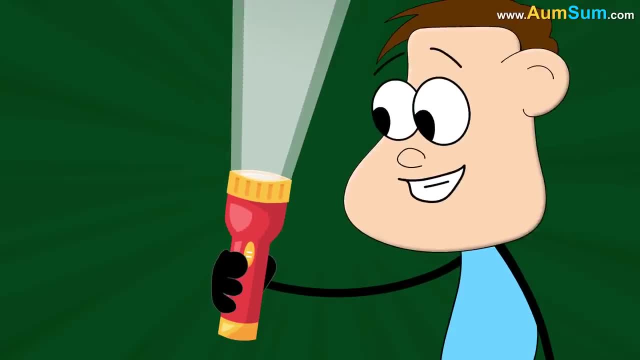 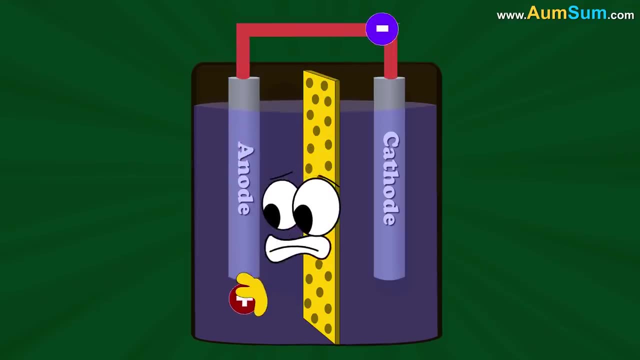 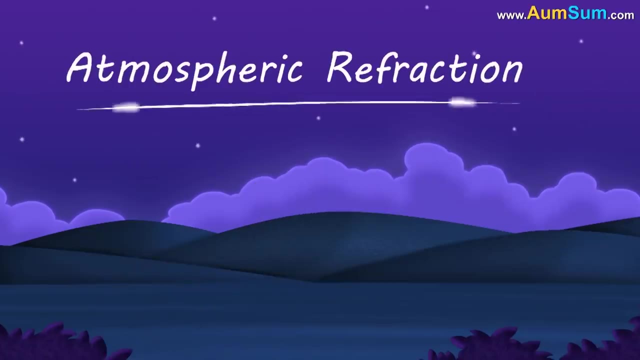 It allows us to power our devices. This is how batteries work. Also, there exists a semi-permeable barrier in the electrolyte So that all the ions do not immediately coat the electrode and thus clog the system. Atmospheric refraction. 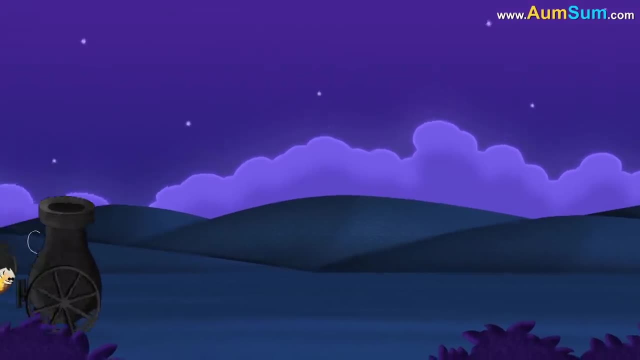 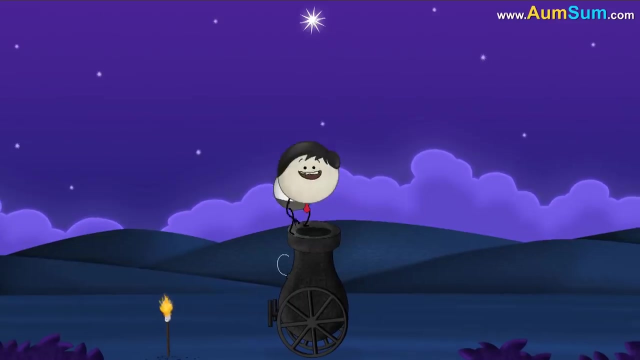 Why do stars seem higher than they actually are? They seem much higher than they really are. They are not made of anything like metals or gas. We have the energy. Our energy has no energy. It just flattens out as it's connected to a beam of light. 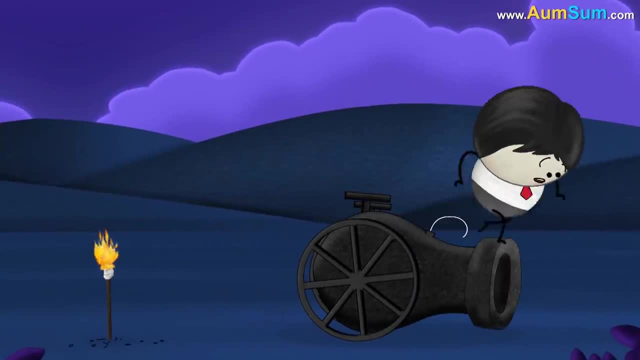 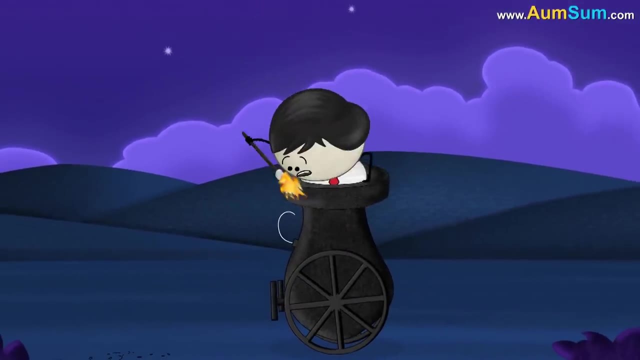 The energy that this beam of light allows us to apply is not exactly the same. It is exactly the same, But the energy that we power our devices up is not the same. As you have understood in this video, our energy is not actually the same. 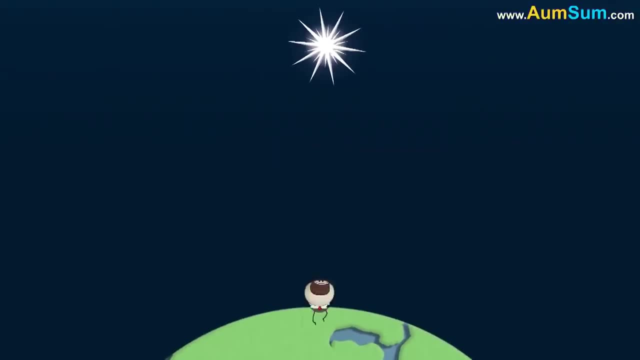 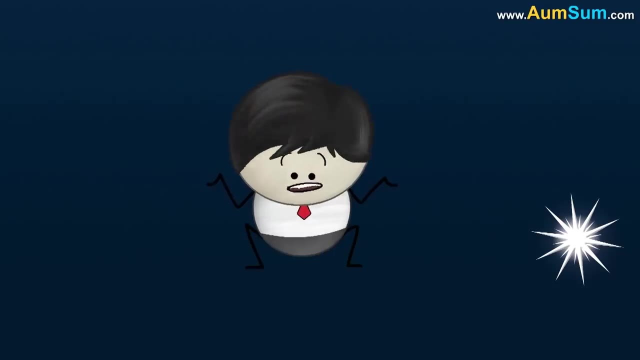 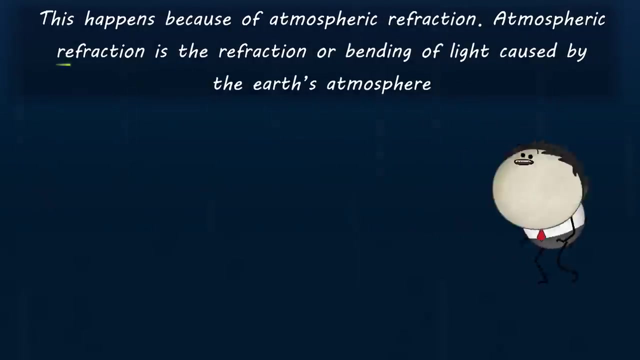 Therefore, the energy we convert to electricity does not compare to the energy that is given to it. The energy that we produce doesn't compare to this energy. Therefore, See, I told you, Do you know why this happens? This happens because of atmospheric refraction. Atmospheric refraction is the refraction or bending of light caused by the earth's atmosphere. It went over your head right? No worries, Let me explain it to you in detail. In the earth's atmosphere, the air closer to the earth's surface is denser due to gravity. 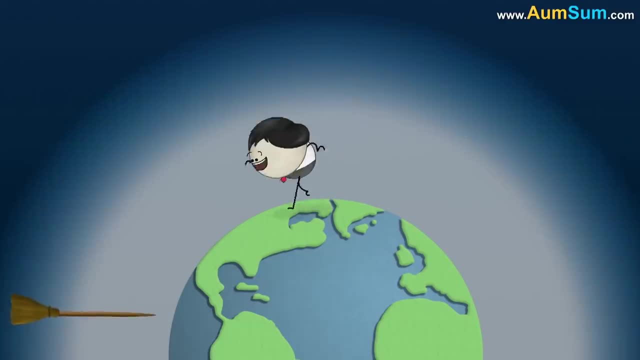 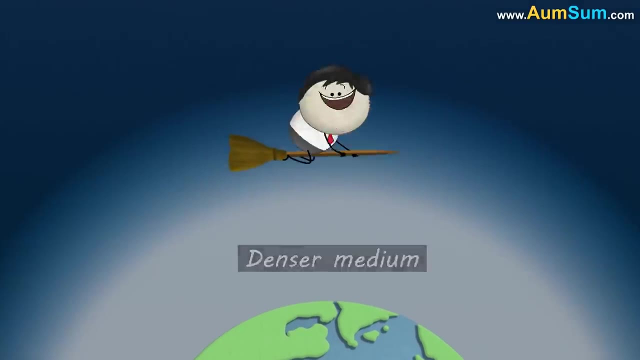 But as we move higher, the air density goes on decreasing. This forms different media of air. The layer of air closer to the earth's surface forms the denser medium, While the layer of air higher up in the sky forms the rarer medium. 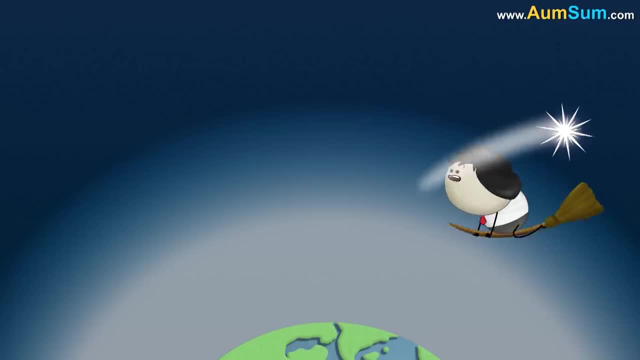 Now, when the light of a star enters our atmosphere and passes from one medium to another, Atmospheric refraction takes place and the light bends. When this light reaches our eyes, our eyes trace it backward as a straight line. Due to this, the light appears to come from a higher point. 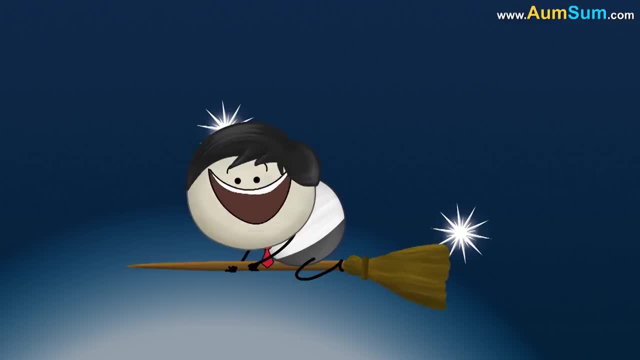 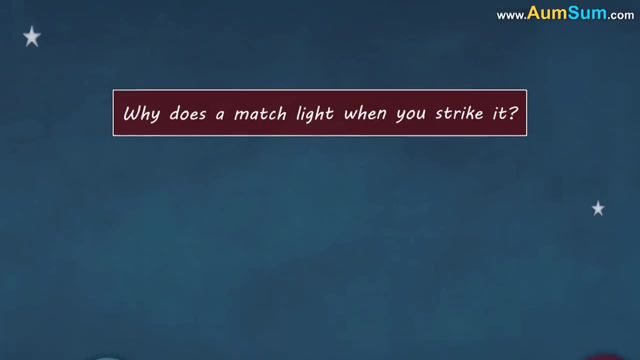 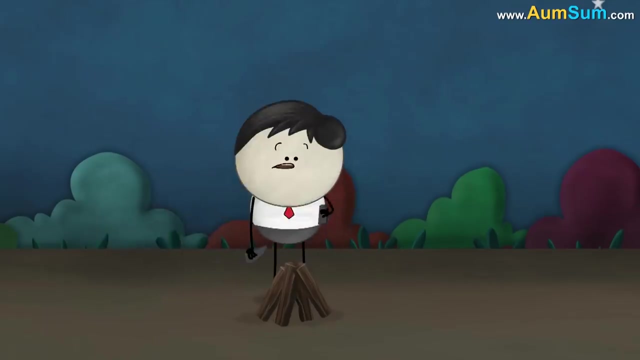 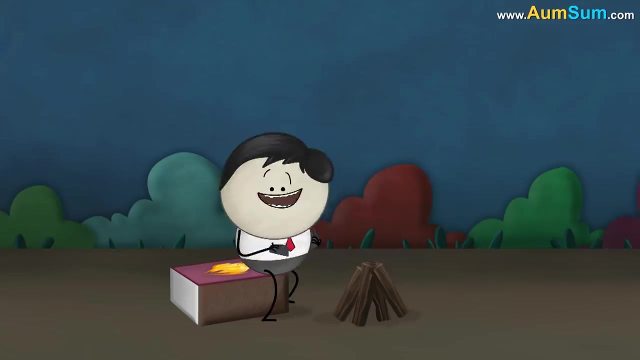 Hence the star seems to be higher than it actually is. Ignition temperature: Why does a match light when you strike it? Why don't you use a match instead? You will be able to light the bonfire easily. No, I don't believe you. 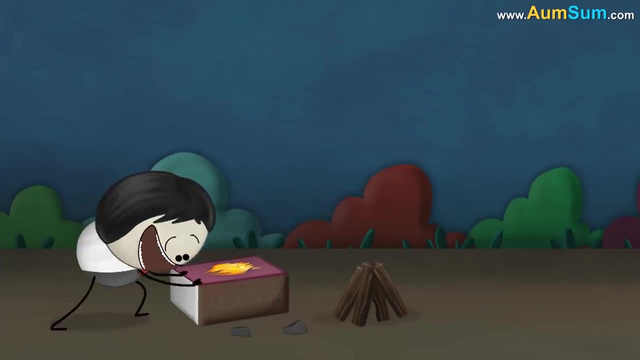 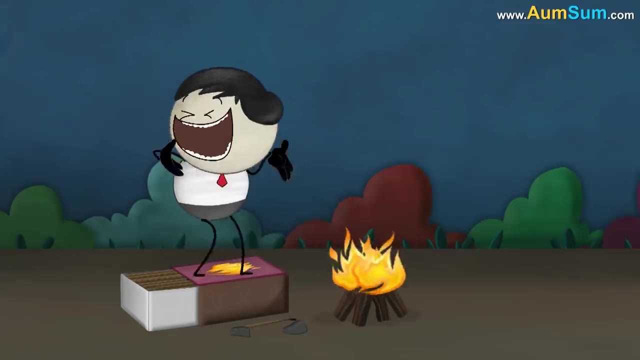 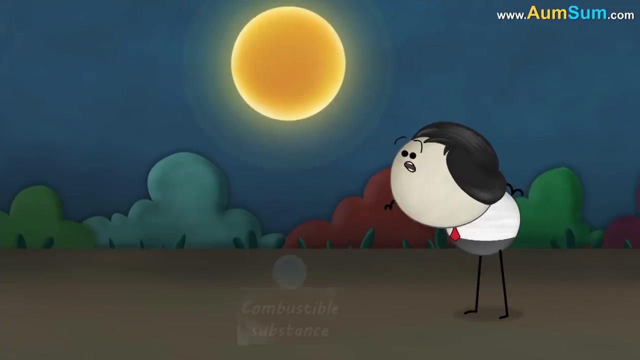 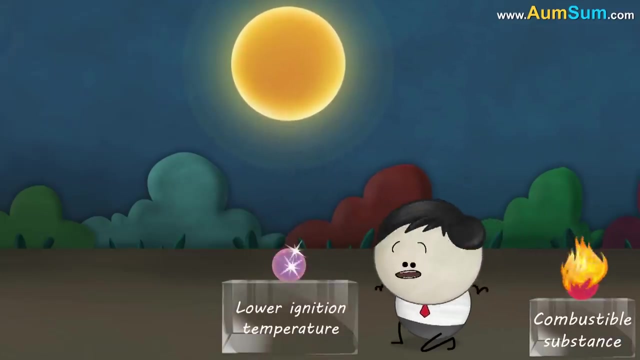 Try it. Look, I told you, Dude, That was awesome. This happened because of low ignition temperature. Ignition temperature is the lowest temperature at which a combustible substance starts burning. Lower the ignition temperature, more easily will it catch fire. 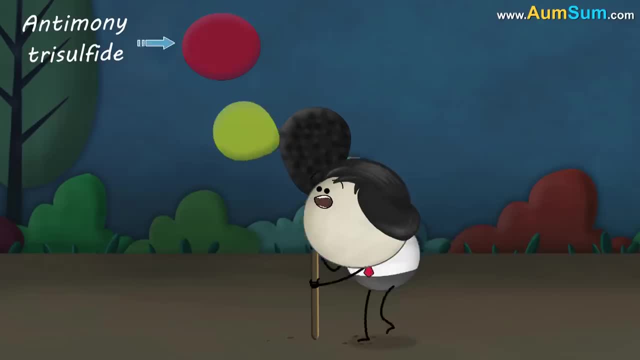 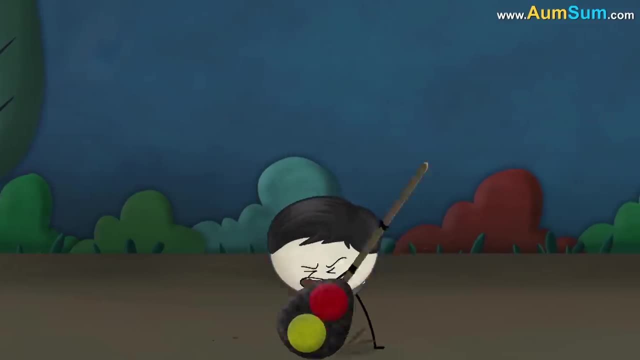 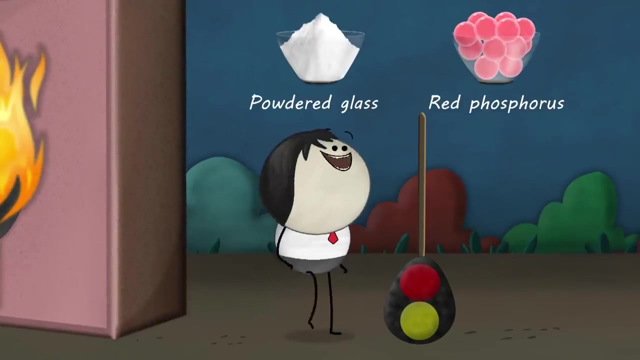 Now. a match head contains antimony tri-sulfide and potassium chlorate Enough. I know how to use it now. No, The match will not light on any surface. The rubbing surface of a match box has powdered glass and red phosphorus.